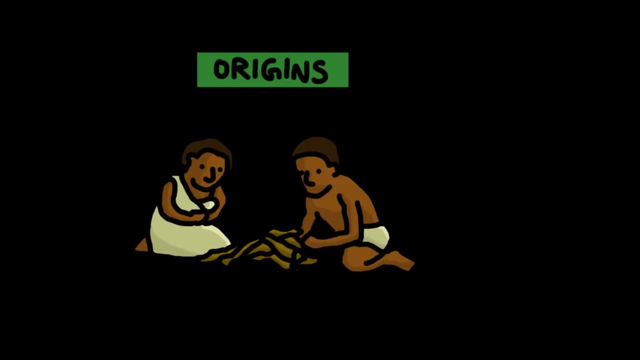 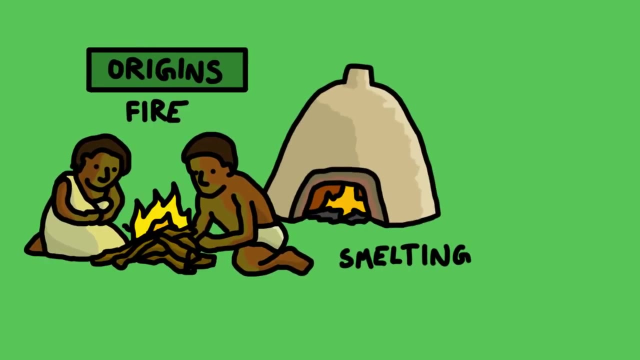 be what we are today if it was not for the chemical reaction of fire. We use this to develop this chemical-reacting object for our own biology and chemistry. We use it to develop other chemical techniques from cooking food, making metal from ores or making glass. 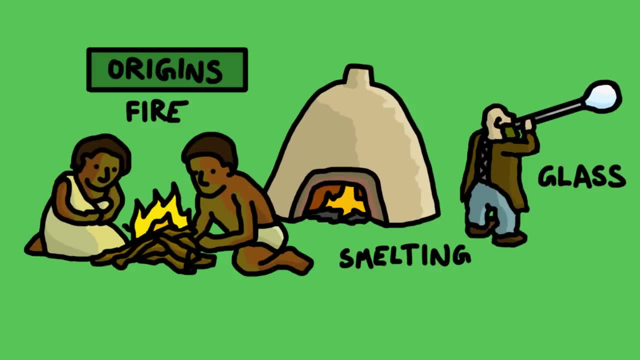 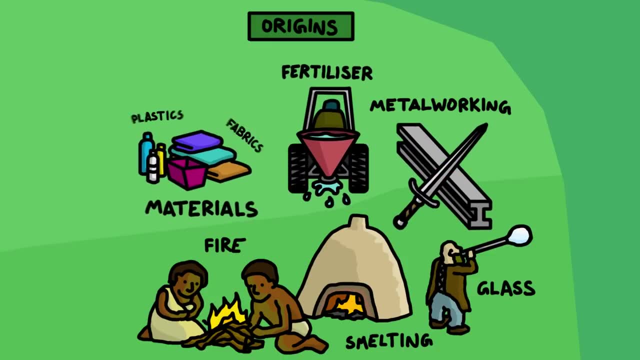 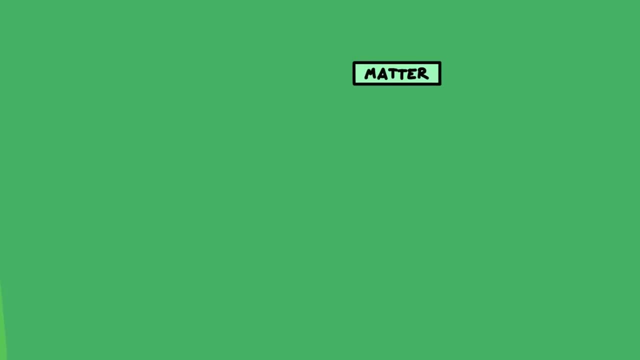 amongst many others. Since then, many advances in human civilisation have been built on the back of advances in chemistry, like metalworking or manufacturing fertiliser, or making new materials and drugs. Let's look at what falls under the umbrella of chemistry. First, there's matter and all the different things that matter is made of. 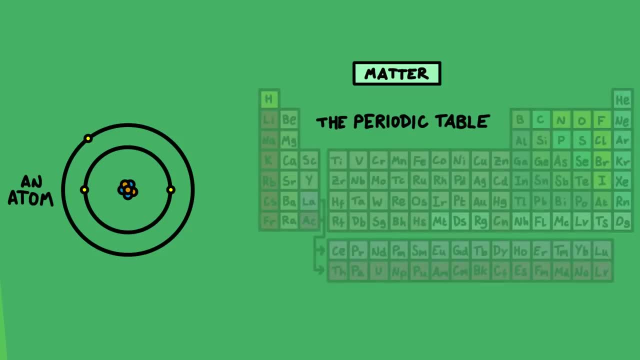 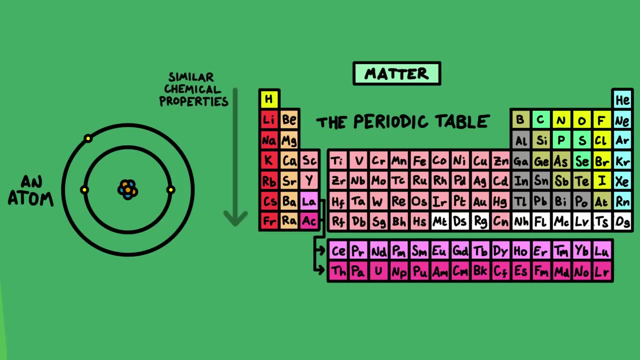 At the very smallest scale. we start with atoms and the periodic table that organises all of the different types of atom called chemical elements. Elements in each column have similar chemical properties. Atoms are made of protons and neutrons in the nucleus, with electrons surrounding them. 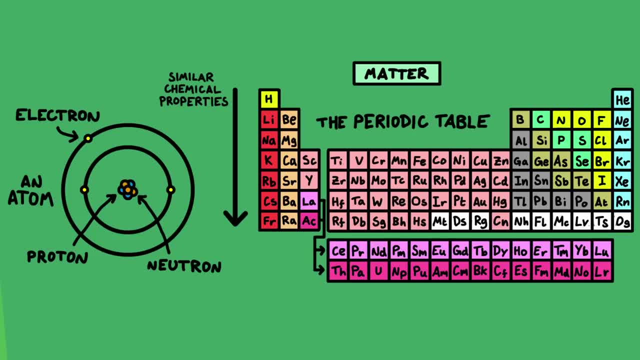 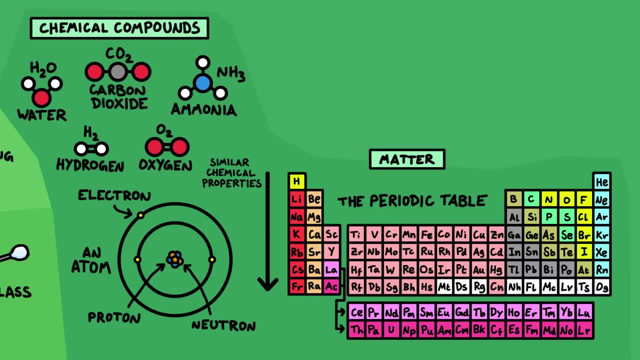 and most of chemistry is due to how these electrons behave. By joining together atoms, you get molecules, and different kinds of molecules are called chemical compounds. Chemical compounds usually have very different chemical properties to the elements that they're made from. Think about it. 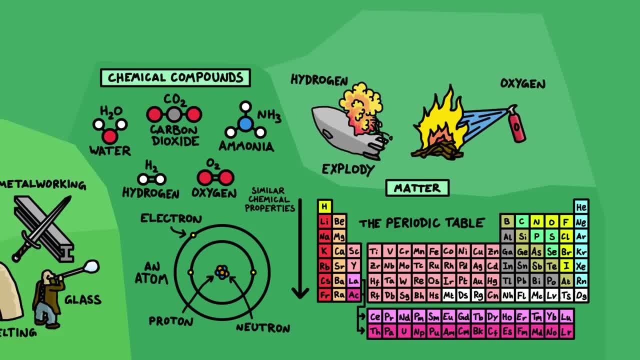 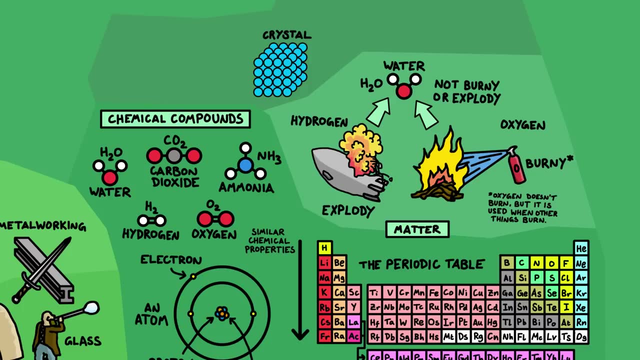 Hydrogen is very exploding. Oxygen is very burny, but combine them together into H2O and you get water, the least explodey burny thing around. Compounds don't have to be made of single molecules. Many solids, like metals or salts, have a crystal structure made of repeating groups. 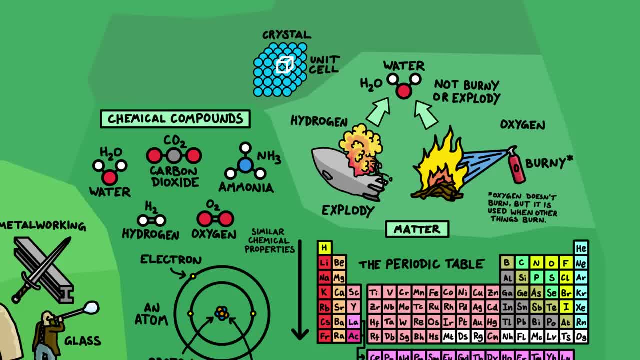 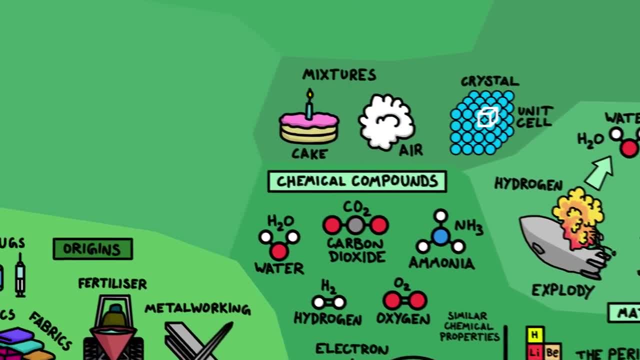 of atoms called unit cells. If you have several substances together, you have a mixture, like the air around you or a cake. Now let's move on to how atoms stick together with a very important subject of bonding. Let's look at how atoms stick together with a very important subject of bonding. 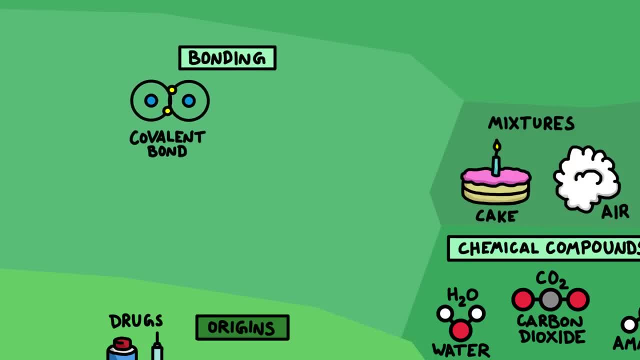 First comes the nuclear. The nuclear is a mixture of the atoms and the neutrons. bonding Atoms bond together in several different ways where they reduce their combined energy by stealing or sharing electrons or moving them into different configurations. A universal rule in science is that everything is always trying to minimise their energy and bonding. 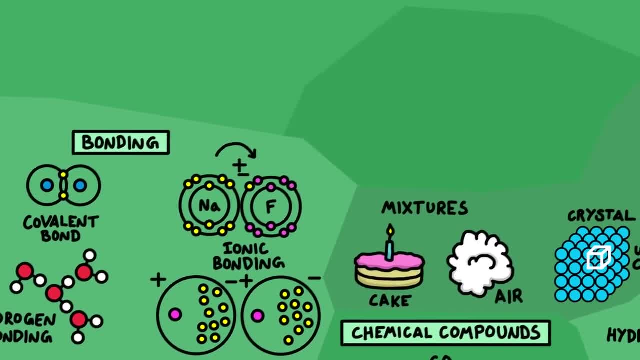 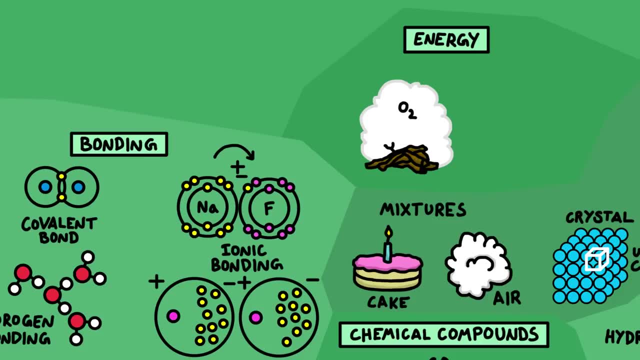 is one way that atoms achieve that. Understanding how energy moves around in chemical substances is vital to understand when reactions will or will not happen. For example, wood won't react with oxygen to start burning spontaneously, but if you give it enough energy to begin with, it will. Another example where energy is very important is where you can speed up. 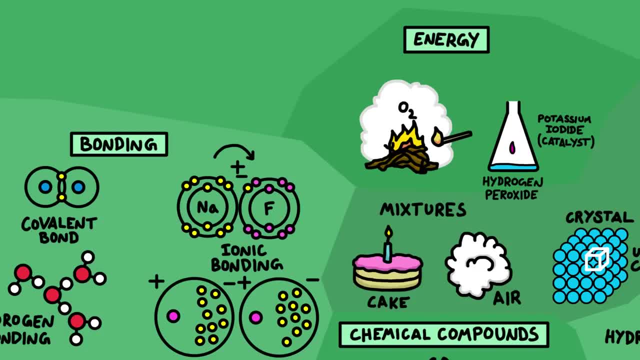 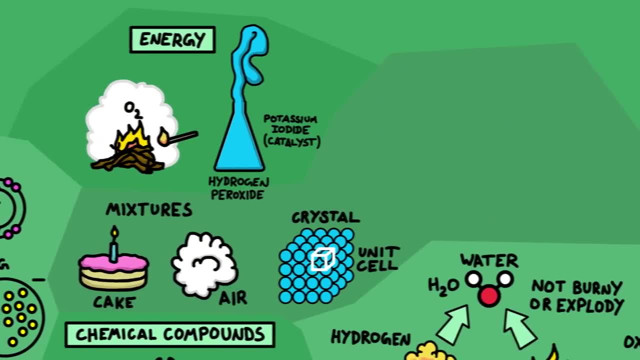 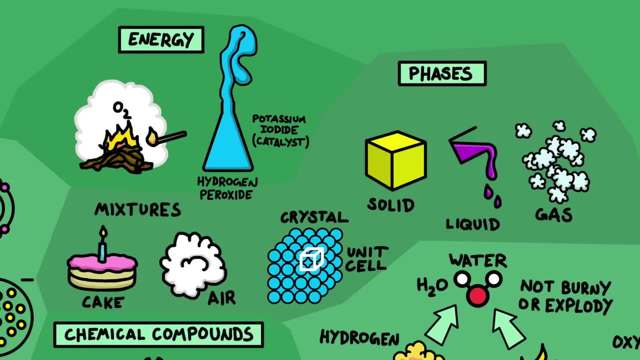 a reaction between two other compounds by introducing a catalyst, and the catalysts make it more energetically favourable and so speeds up the reaction. Energy also determines when compounds will exist in the different forms: solid, liquid or gas. Which form they'll be found in comes from the temperature. 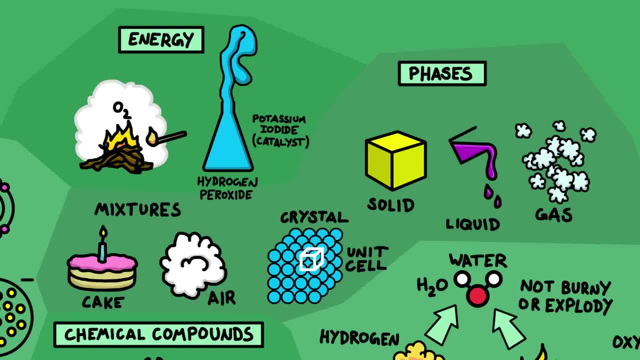 that they're at and the pressure that they're under. The values vary for each material, but in general things are solid at low temperature and or high pressure, and gas at high temperature and low pressure. Another really interesting form of matter is a plasma, which is where 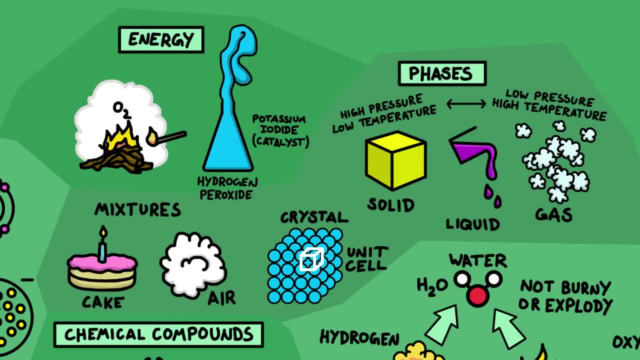 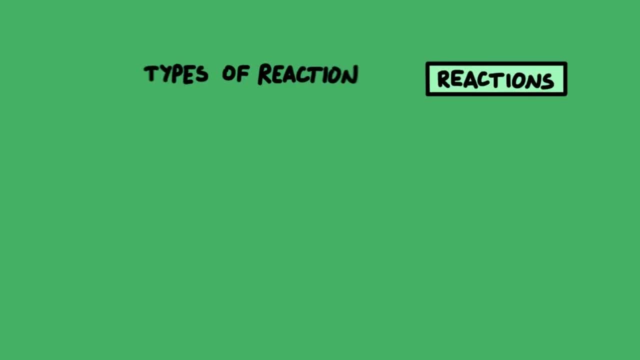 you rip the electrons off atoms in a gas to make them into ions. This is what's used to make neon lights. Chemical reactions form the core of chemistry: Which compounds react with each other, Why they react And what is left over after a reaction. 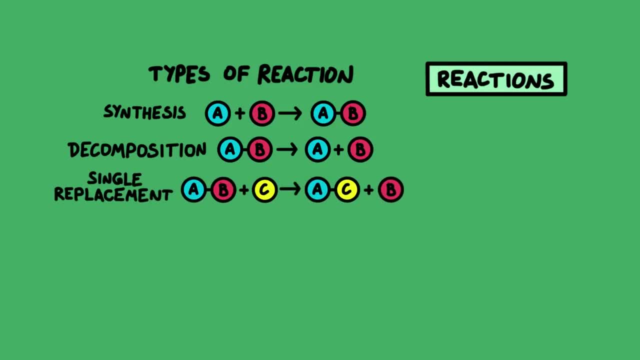 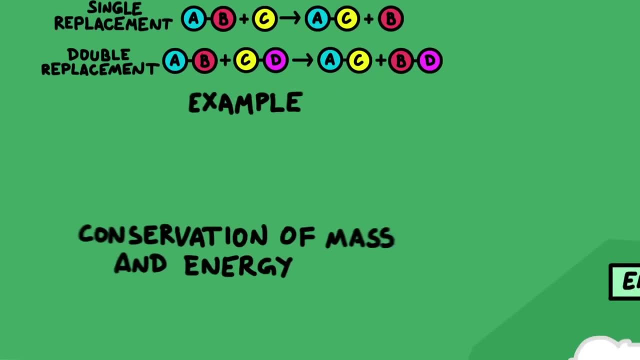 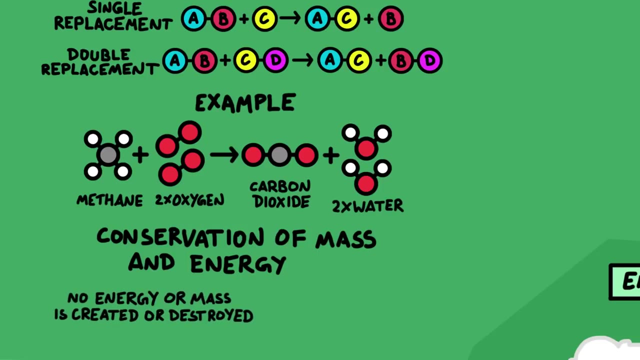 There are many different kinds of reactions, which can be categorised in different ways. All of these reactions are governed by a set of fundamental rules called chemical laws, the foundation of which is the conservation of mass and energy, which means that no matter or energy is created or destroyed in a chemical reaction. They're just changed to different. 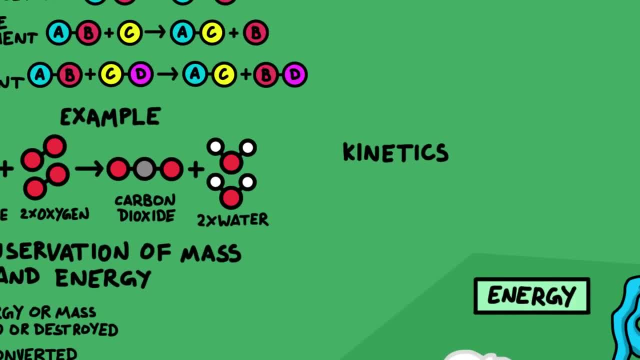 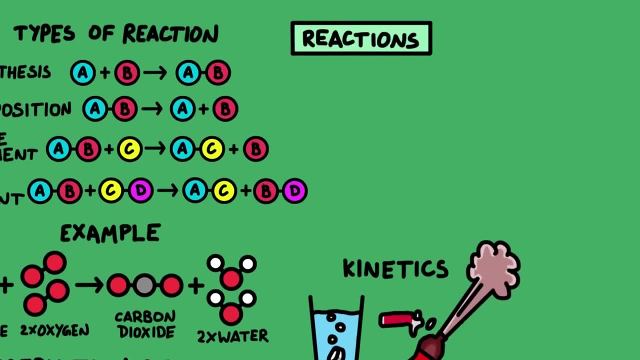 forms. Kinetics is the study of how fast reactions happen and the things that control them. They're what the reaction rates are. A reaction where electrons are transferred from one reactant to another is called an oxidation reduction reaction, or a redox reaction for short. Oxidation means a loss of electrons from a substance and a 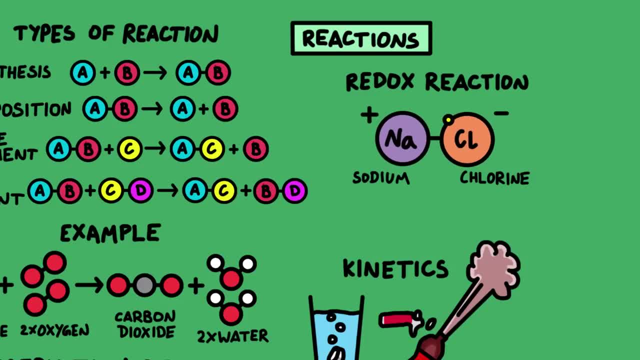 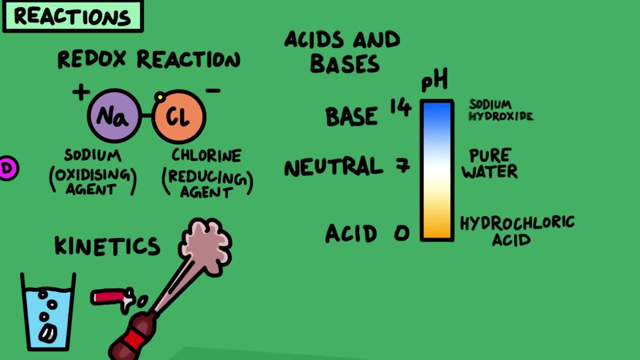 reduction means the gain of electrons, and they have to happen together. An example is sodium and chlorine. Chlorine is the reducing agent and sodium is the oxidizing agent. Another important property of substances is their pH, whether they are an acid or a base. There are several theories to model acid-base. 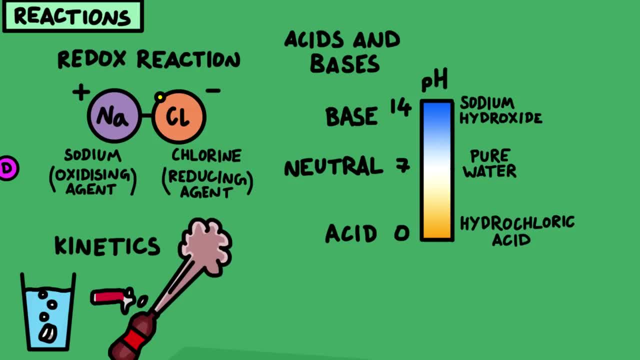 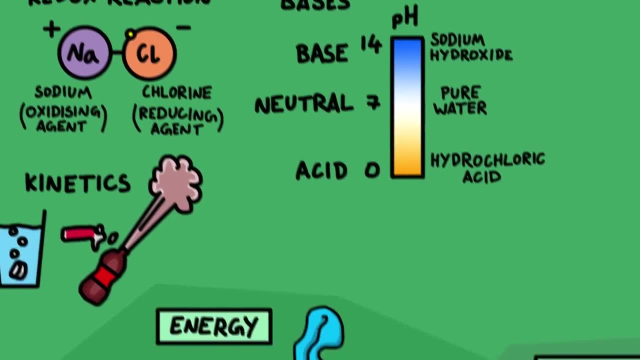 reactions. but one way to think about it is that acids are substances that have a hydrogen ion ready to give up in a chemical reaction and a base is a substance that takes a hydrogen ion. If there are a number of different chemical compounds which can react with each other back and forth, there can be. 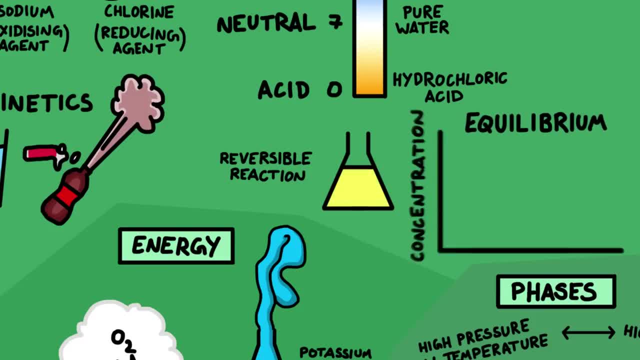 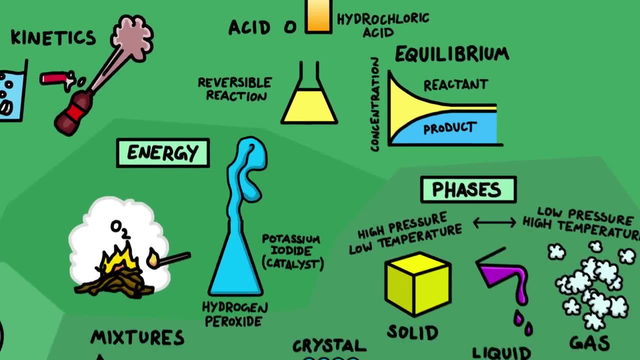 swings between one substance and another. Equilibrium is where the amount of oxygen that goes into an acid-base compound- that is, a amount of each substance- is constant, even though a reaction may still be taking place. This can also happen in phase changes, like from solid to liquid or liquid to gas. 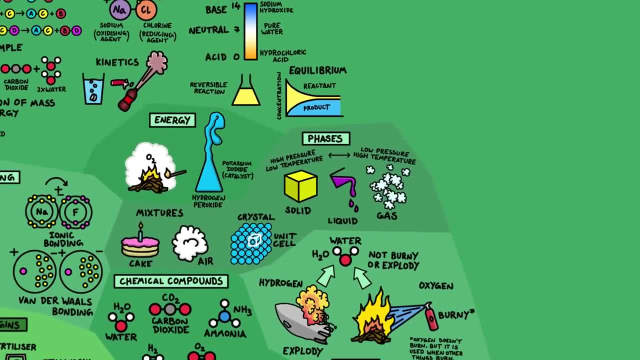 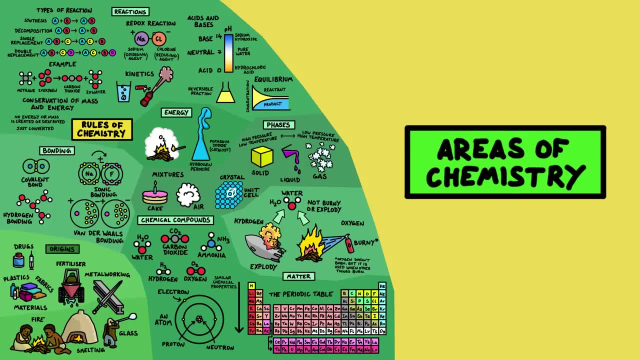 So those are the basics of chemistry. Research in chemistry looks at how these rules apply in different chemical systems. So now I'm going to move on to look at the different fields in chemistry. Theoretical chemistry attempts to explain the structures of atoms and molecules, and 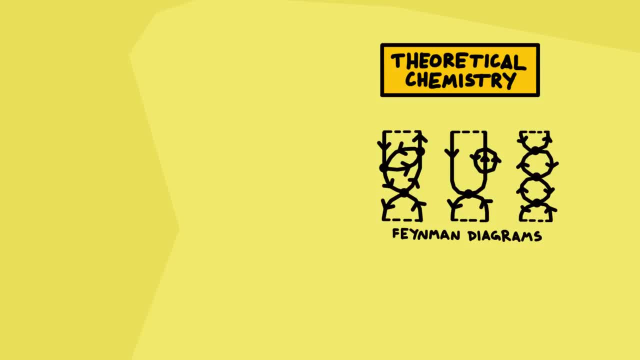 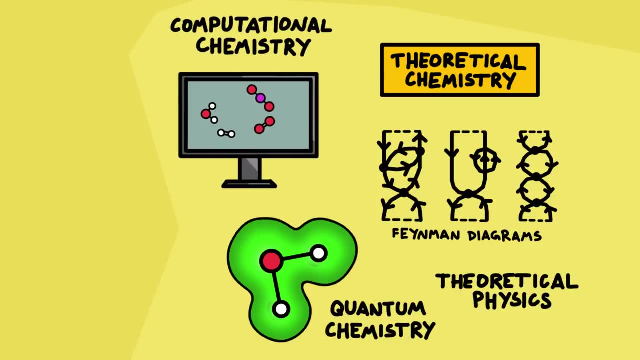 how they interact using mathematical methods. It's very closely related to theoretical physics and quantum chemistry and often uses techniques in computational chemistry, where atoms, molecules and reactions are simulated in a computer, Simulating the proper quantum behaviour of anything more complicated than a single hydrogen. 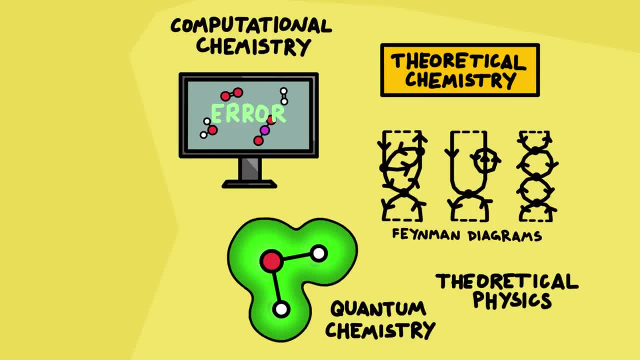 atom is very difficult for multiple bodies, So many cutting edge techniques in computer science are used to try and simulate molecules and how they interact with each other. In fact, this is one of the most exciting applications of quantum computers, because they'll be able to directly simulate chemical systems and will help with things like discovering 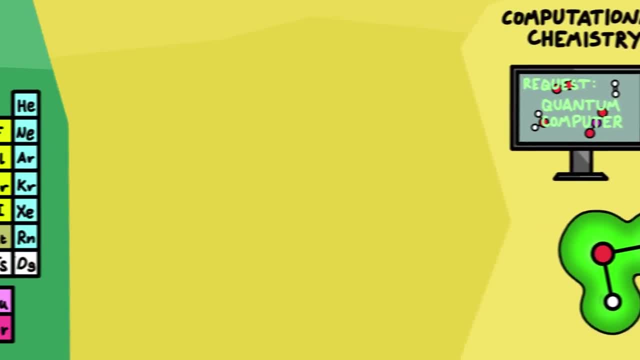 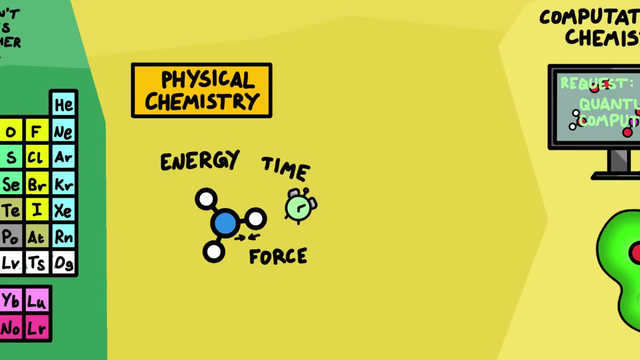 novel materials and drugs and a whole lot more. Physical chemistry studies chemical systems in terms of their physics, so things like energy, force, time, motion, thermodynamics, quantum properties, amongst others. There are many sub-fields like looking at the electronic properties in electrochemistry. 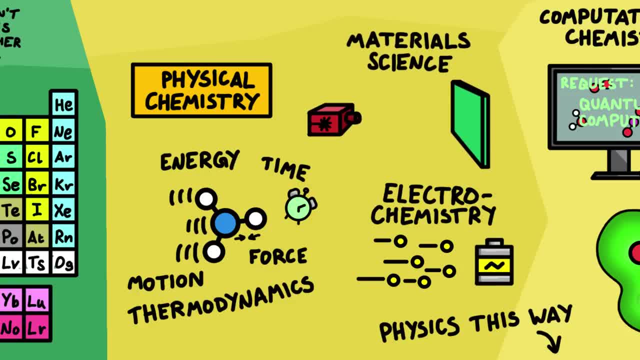 quantum physics, quantum physics and quantum physics. It's also important for developing better batteries- or material science, which is trying to create materials with new properties like extreme strength, durability or self-healing. This is a critical problem with building earth-based nuclear fusion reactors which are reliant on. 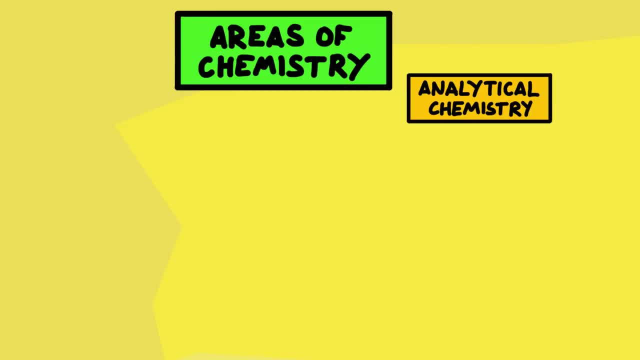 new materials. Analytical chemistry is like detective work: You've got a sample of something and you need to work out what it's made of and the amount of the different components. Chemists could measure different properties of different materials. Traditional techniques involve wet chemical techniques like precipitation, which separates 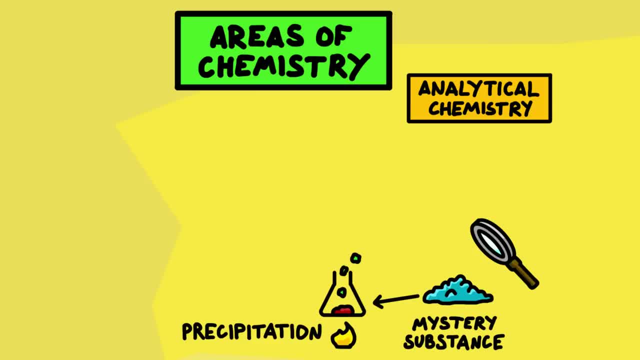 compounds depending on what temperature they evaporate. There's also a huge array of modern techniques, like chromatography, where different compounds move at different speeds through a solution and so separate, Or the many different kinds of spectroscopy that can detect materials by shining light on them, or mass spectroscopy, where the materials are flung through electric or magnetic fields. 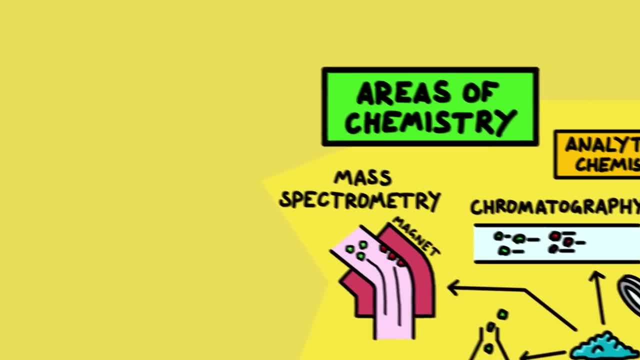 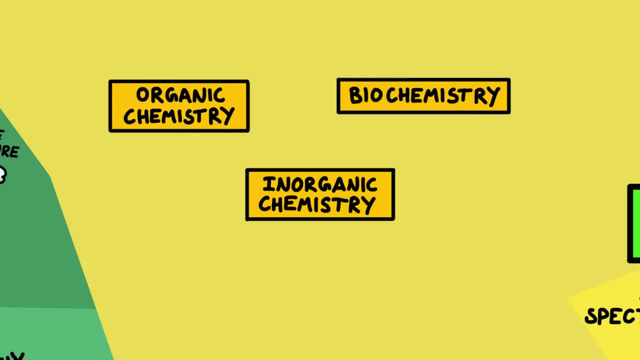 to separate them according to their masses. And finally we get to the huge fields of inorganic, organic and biochemistry. Organic and biochemistry look at the chemistry of living things, and inorganic chemistry looks at everything else, although there is still a large amount of crossover. 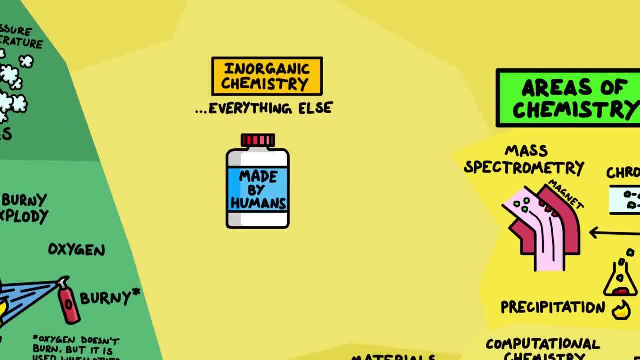 Most of the inorganic compounds that are studied are man-made, and a lot of the motivation is to find chemicals with new properties that can be used in the chemical industry. in the wider world, In fact, there are very few areas of human endeavour where inorganic compounds can be used in the chemical industry. It's almost. 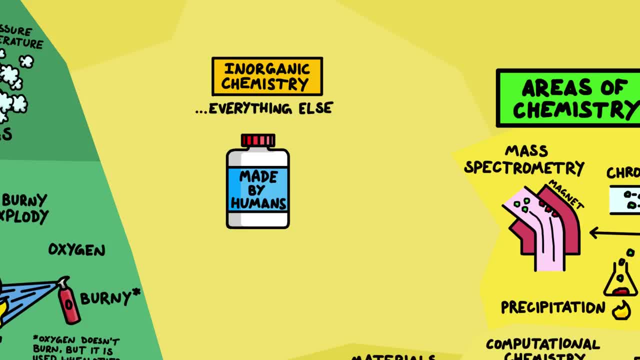 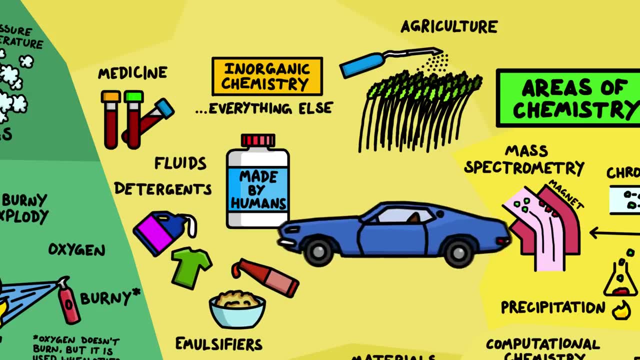 impossible to find a single component or chemical compound that can make a difference in physical organic chemistry has not been used in some way. There's medicine and agriculture, special fluids like detergents or emulsifiers, special coatings, materials, pigments or fuels for. 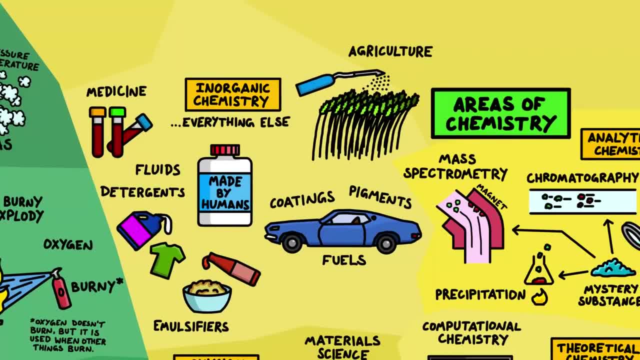 many industrial purposes. Within chemical production itself, catalysts are very important as they speed up other chemical reactions. Inorganic chemistry also bleeds into material science, making solids with novel crystal structures like high-temperature superconductors, for example. The list is endless. 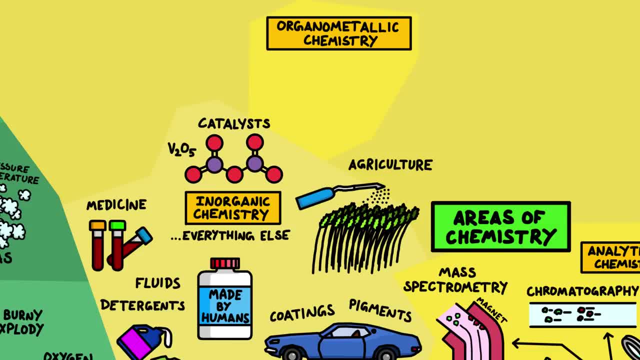 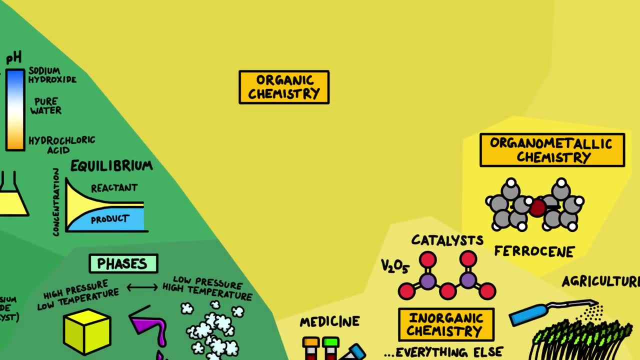 Between inorganic and organic chemistry sits organometallic chemistry. This looks at organic compounds which are bonded with a metal and are typically used in reactions in the chemical industry, often as catalysts. Organic chemistry looks at the structure and behaviour of the molecules of life, which 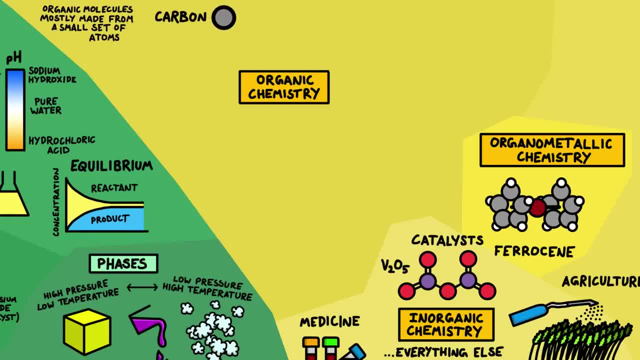 are typically built from a small set of different atoms – carbon, hydrogen, oxygen and nitrogen, plus a few others. Organic chemists also look at making new organic compounds with useful properties. Organic molecules all contain carbon, and the carbon-hydrogen bond is the most common. 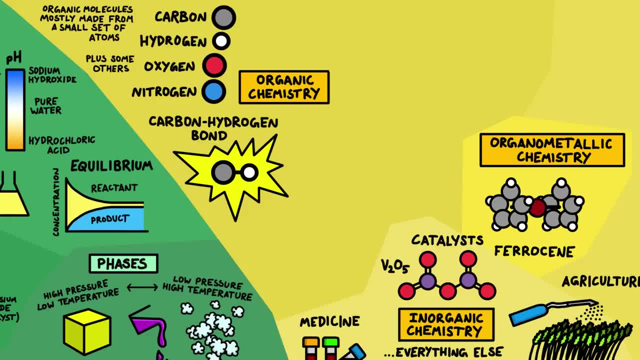 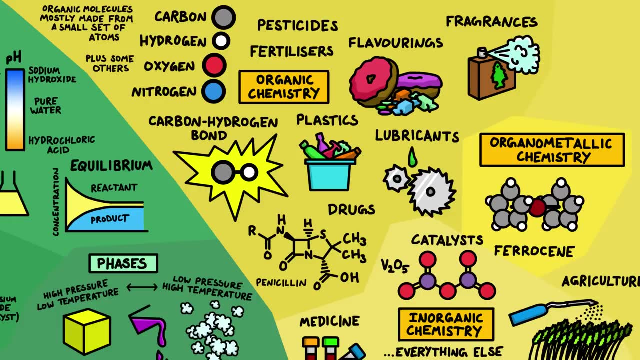 structure in organic chemistry. There are a huge number of applications of organic chemistry in industry – fertilisers, pesticides, lubricants, polymers and plastics. And in the consumer world. there's fragrances, flavourings and preservatives and, of course, drugs in the pharmaceutical industry. 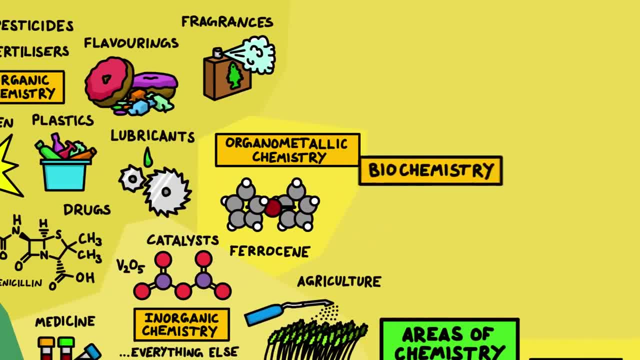 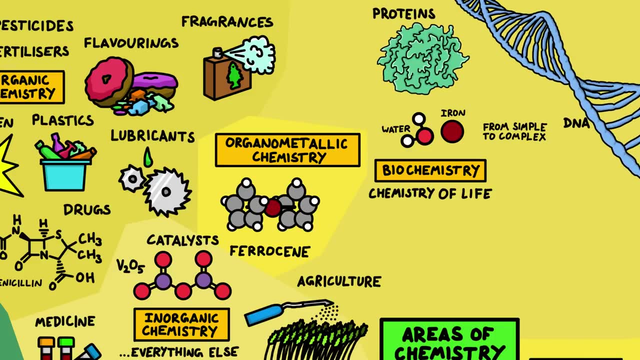 Ingredients. And finally, out of organic chemistry comes biochemistry, which studies the chemistry of living organisms. Biochemistry studies components that can be inorganic, like water or minerals, but also looks at the biggest and most complex molecules, like proteins, fats and DNA.